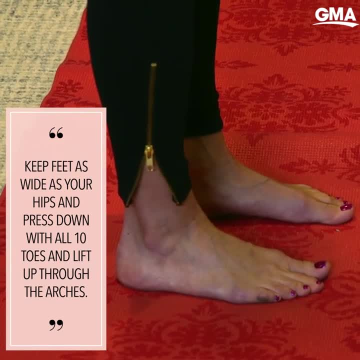 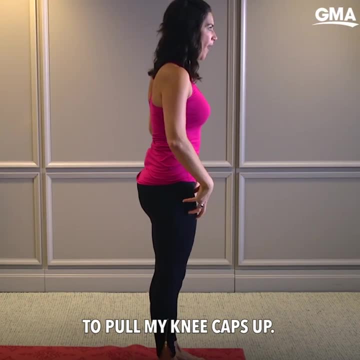 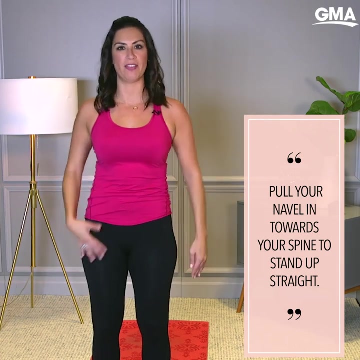 foundation. my feet are as wide as my hips. I'm pressing down with all 10 toes and lifting up through the arches. Then I'm squeezing my quads to pull my kneecaps up, pulling my belly button, navel in towards my spine to stand up even straighter and support my low. 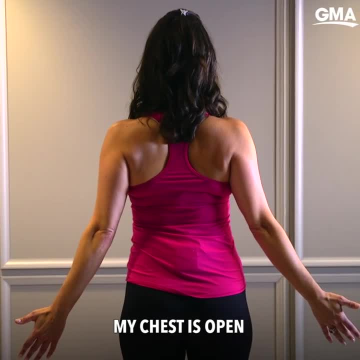 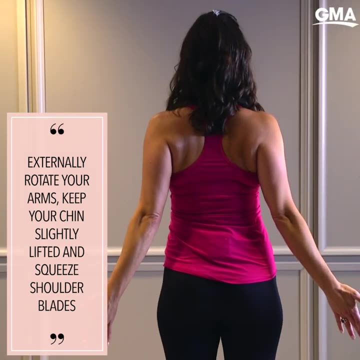 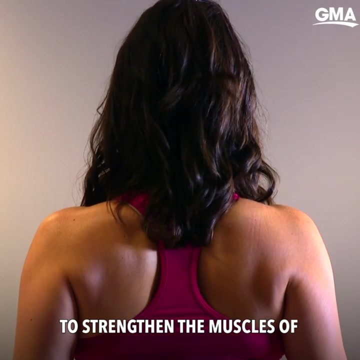 back And then my shoulders are back, my chest is open and my arms are externally rotated. My chin is slightly lifted and I'm squeezing my shoulder blades together in my upper back so that I can open my chest but also to strengthen the muscles of my upper back. From mountain pose we're going to reach the arms out. 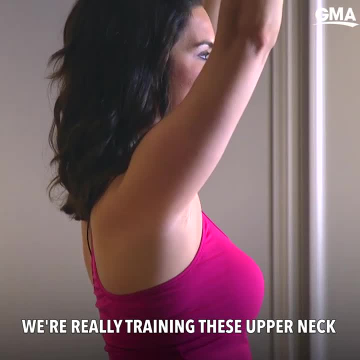 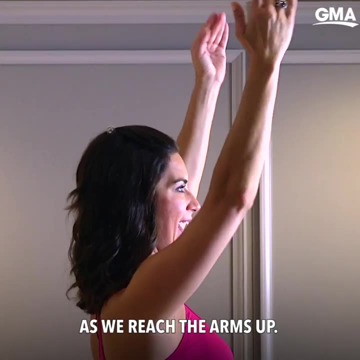 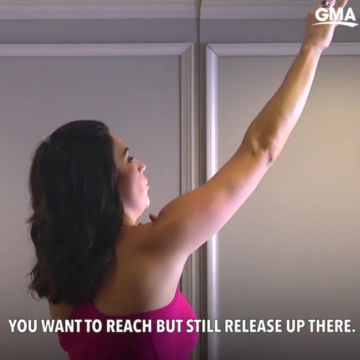 to the sides and up as you breathe in. We're really training these upper neck and these upper back muscles to relax as we reach the arms up. So if you're reaching for things throughout the day, you want to reach but still release up there. So as we have the arms up, we relax the shoulders down. 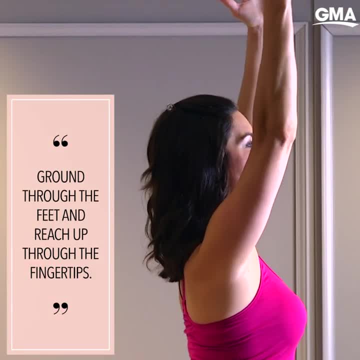 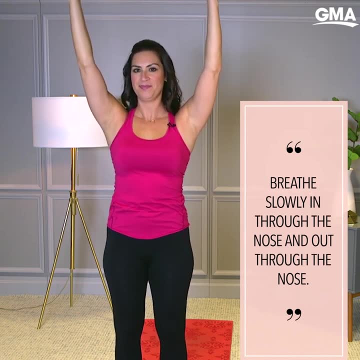 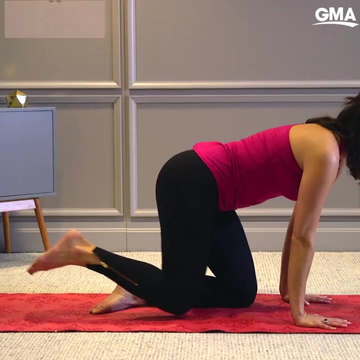 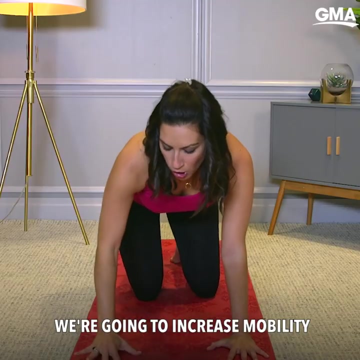 we ground through the feet and reach up through the fingertips and breathe slowly In through the nose and out through the nose. Now let's come down onto our hands and knees- for cat and cow. So lining up the wrists directly underneath the shoulders and the knees directly underneath the hips. We're going to increase. 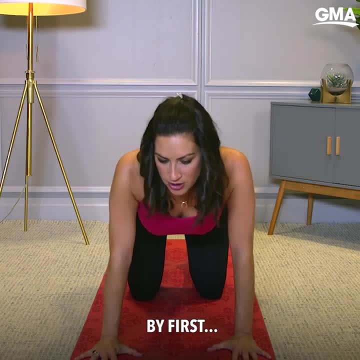 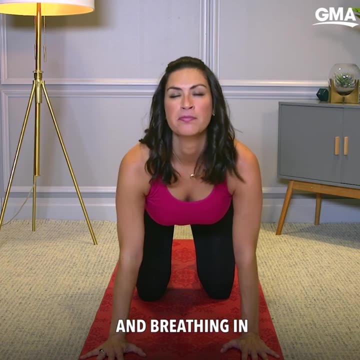 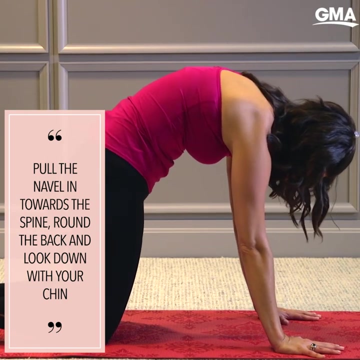 mobility in the upper, middle and lower spine by first bringing the shoulders back and lifting the head up and sticking the tush back and breathing in, And then we do the reverse: Pull the navel in towards the spine, round the back and look down. 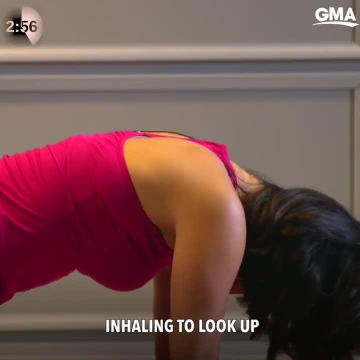 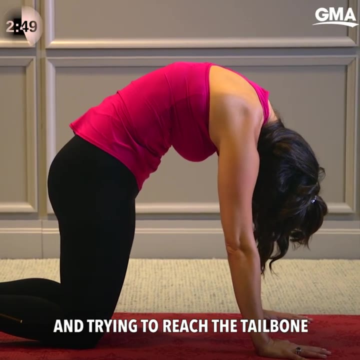 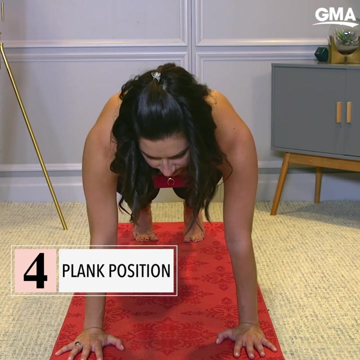 with your chin and your chest, Inhaling to look up, sticking the tailbone back behind you and then exhaling to round down and trying to reach the tailbone down towards the ground From your hands and knees. now we're going to move into a plank position, So we're going to walk the 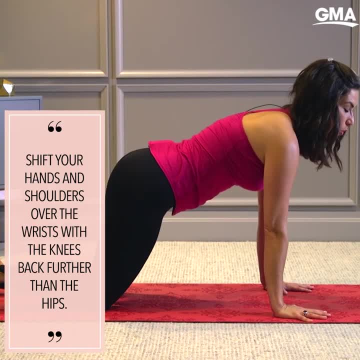 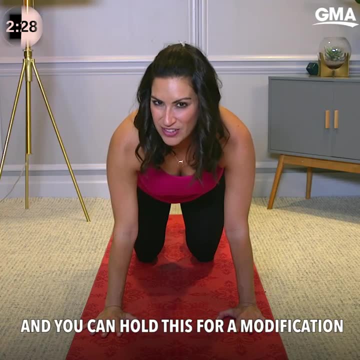 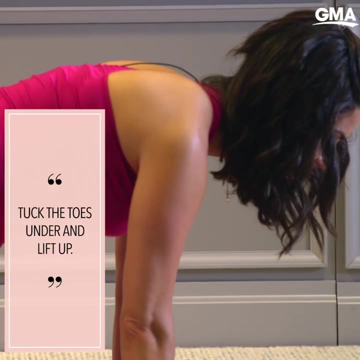 hands forward just a couple of inches and shift the shoulders forward over the wrists, with the knees back further than the hips, And you can hold this for a modification. with your abs drawn in For full plank, tuck the toes under and lift up, Then, looking down just a couple of inches in front of you, breathe here. 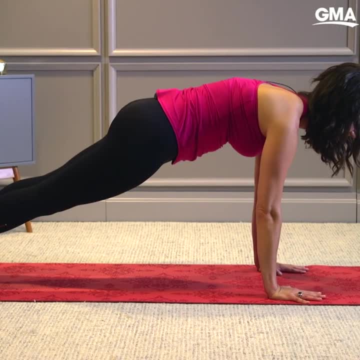 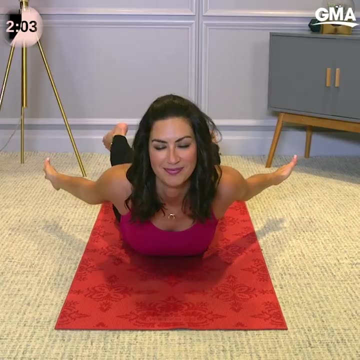 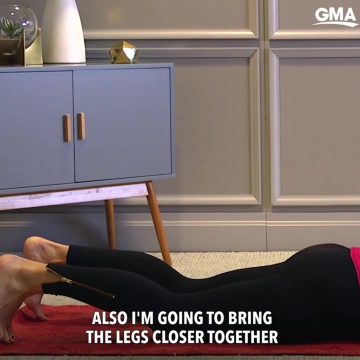 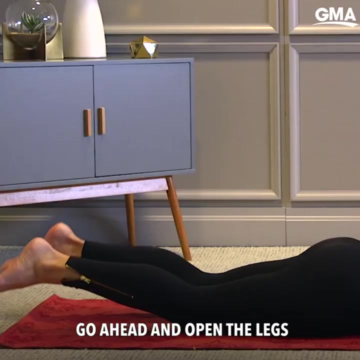 Another great pose for posture is locust pose, Coming down onto your stomach. make sure that you pull your navel in towards your spine. Also, I'm going to bring the legs closer together, but if you have blowback issues or need a modification to make this a little bit easier, go ahead and open the legs as wide as the hips. I'm going to. 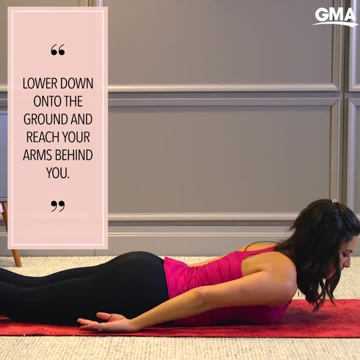 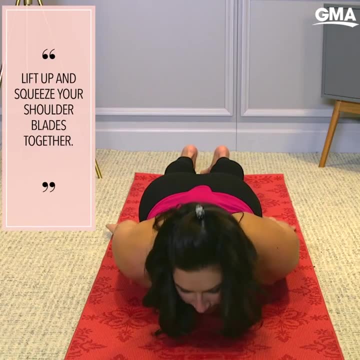 lower down onto the ground and reach my arms behind me. so from this position you can start with your forehead on the mat and your shoulders resting down. as you lift up, the shoulder heads are going to lift up as well. the upper back squeezes together, squeeze. 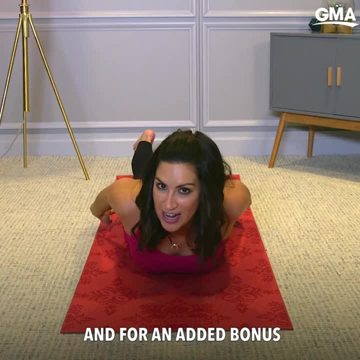 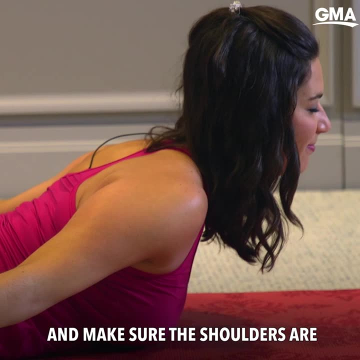 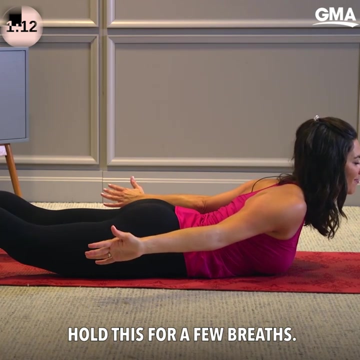 your glutes and then lift the legs up. and, for an added bonus, since we're working on posture, you can open the palms, open the legs as you lift up and make sure the shoulders are pulling down instead of hunching up towards your ears. hold this for a few breaths. 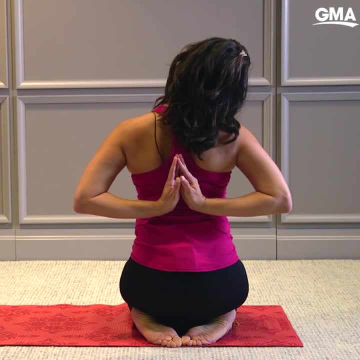 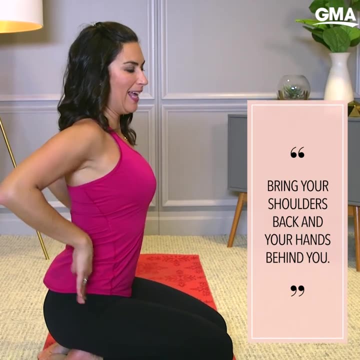 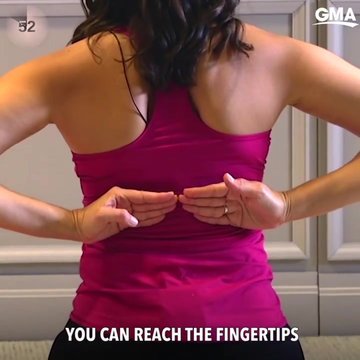 reverse prayer is a great yoga pose that will help to open up the chest and it feels really good too. first we're gonna bring the shoulders back and then bring the hands behind you. now, if you're a little bit tight, you can reach the fingertips towards each other here and just bring the elbows and the shoulders. 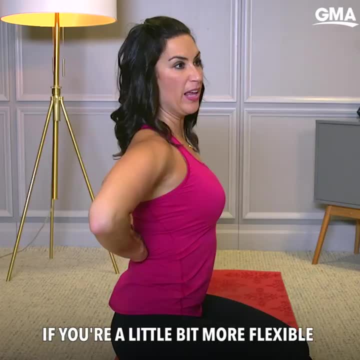 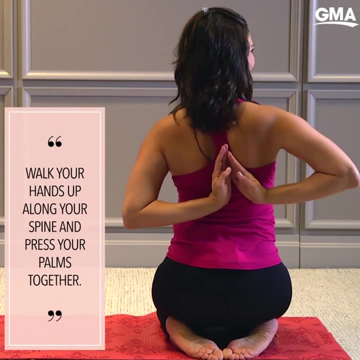 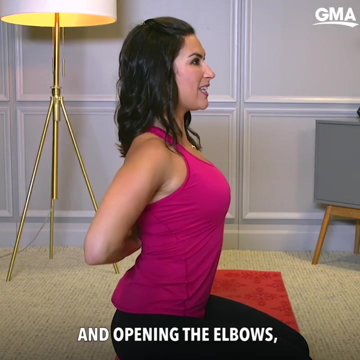 back and this will be your reverse prayer position. If you're a little bit more flexible and open in the shoulders, then you can go into full reverse prayer, So walking the hands up along your spine in between your shoulder blades and then pressing your palms together and opening the elbows, opening the chest, but pulling the navel in. 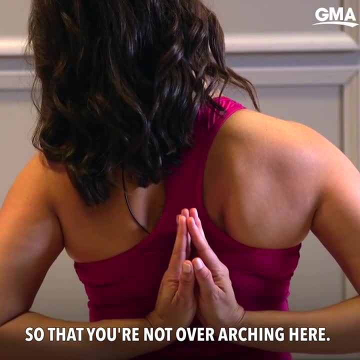 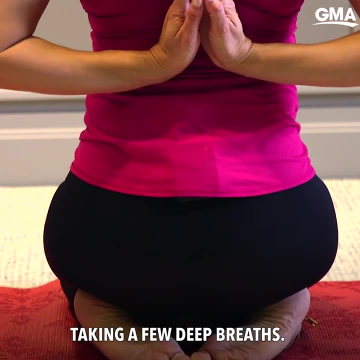 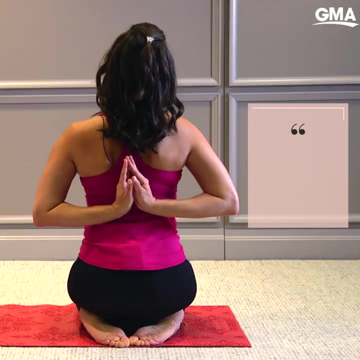 towards the spine so that you're not overarching. here We're pulling the navel in, shoulders are back and chest is lifted, Doing this here and taking a few deep breaths. For an added bonus, you can stretch along the sides of your neck by dropping one ear. 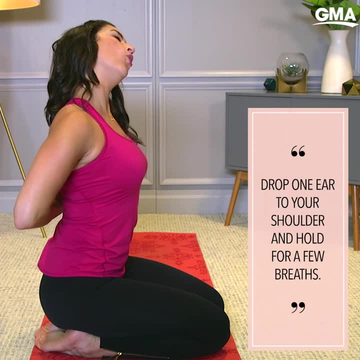 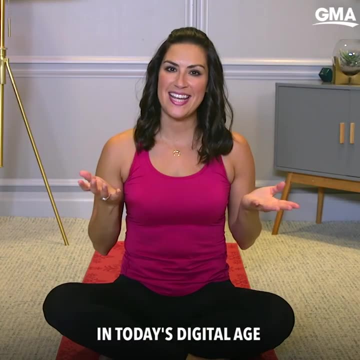 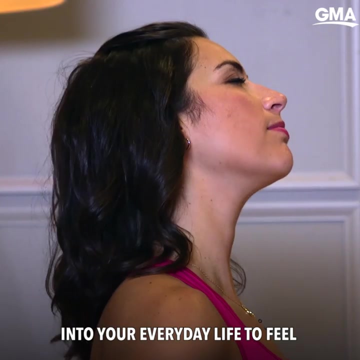 to that same shoulder, on the same side, holding for a few breaths and then coming back to center and going to the other side. In today's digital age, having poor posture is pretty inevitable, So step it up and integrate these yoga poses into your everyday life to feel instant relief. and relaxation Namaste.